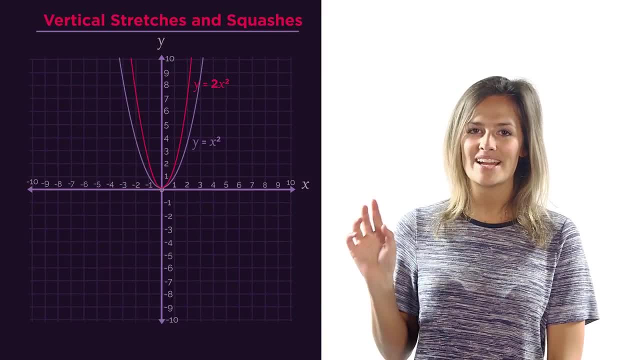 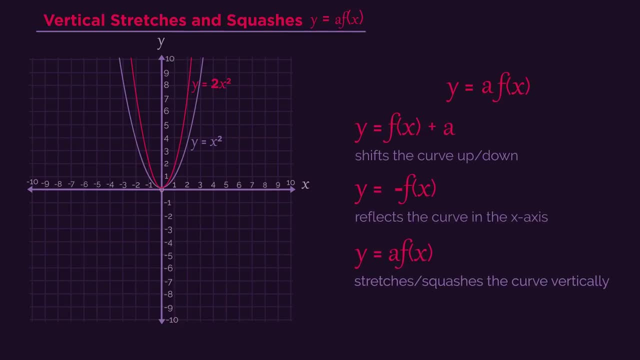 to its changed shape. Let's start with vertical stretches and squashes, as they're a little easier. As with all vertical transformations, we apply the transformation to the whole function. so the outside See how the number goes here, If it's a 2,, a 3 or any number bigger than. 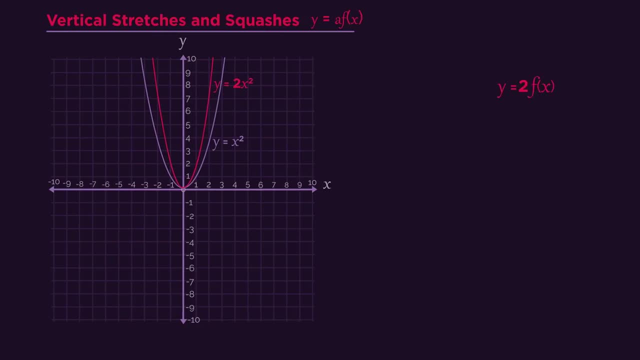 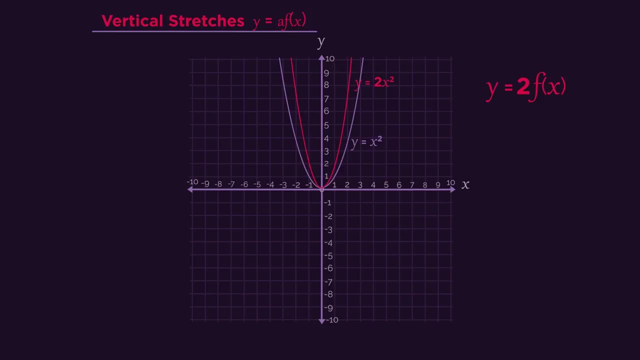 1, the curve will be stretched. So, because this curve has the equation y equals 1, the curve will be stretched. So, because this curve has the equation y equals 1, the curve will be in the shape of a 1.. The 2 means we need to double every y value Here. 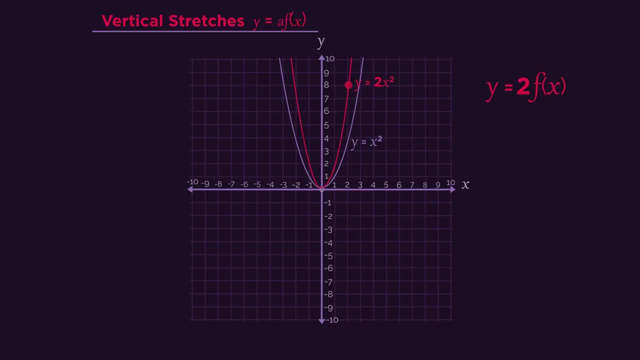 4 needs to double to 8, so every y coordinate doubles in size. If the new curve was: y equals 3x squared, then every y coordinate would need to multiply by 3.. So 1 goes to 3, and so on. See what happens when the equation is: y equals a half x squared. 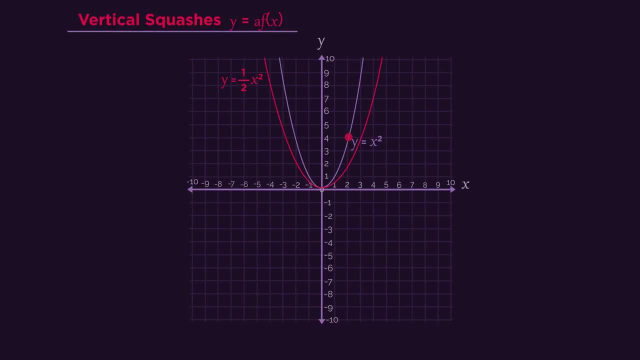 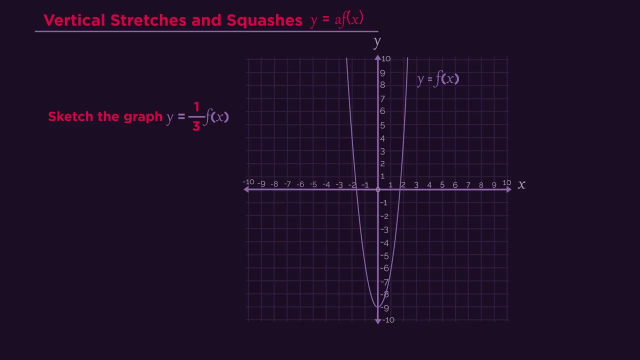 x squared The y coordinate's half in size, so four goes to two. If you have to transform a graph yourself, just take it point by point. So we have the graph of y equals f of x and we need y equals a third f of x. So we divide each y coordinate by three. Negative nine moves to negative three. 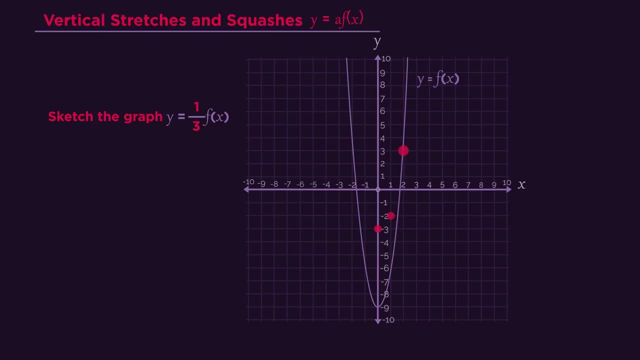 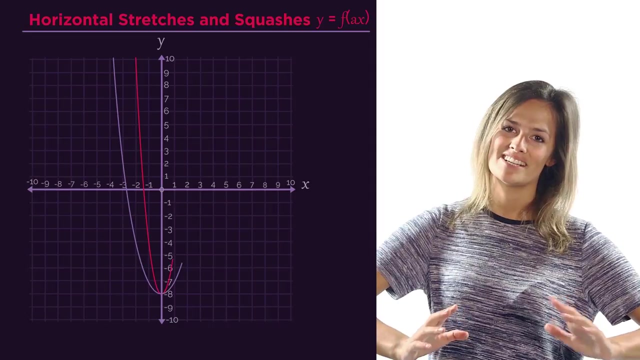 Negative six goes to negative two, Three goes to one and you'll end up with your transformed graph. So y equals a third f of x would be squashed vertically by a third. Horizontal stretchers and squashers aren't much different, As with all horizontal. 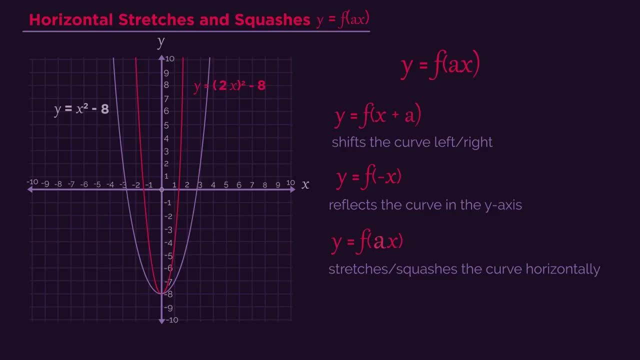 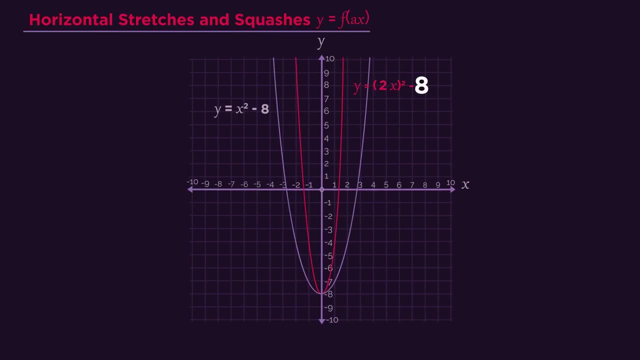 transformations. we apply the transformation directly to the x's. See how the two just goes with the x's X and ignores the eight. Notice how two seems to squash the curve horizontally, whereas a half stretches the curve As with all horizontal transformations.